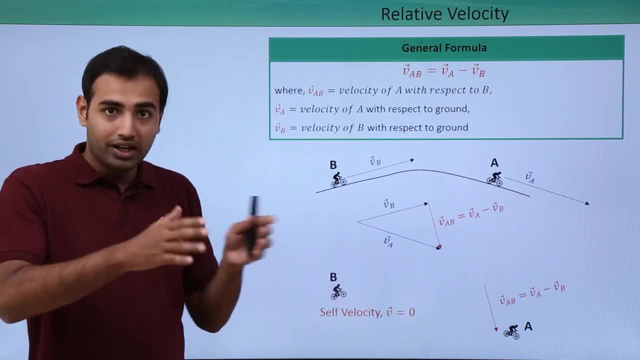 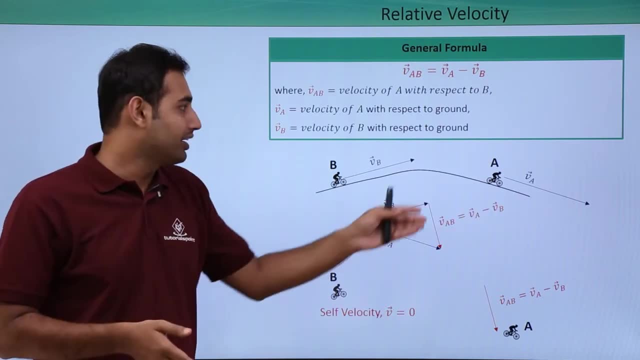 of velocity of A with respect to B. So if you are an observer instead of B, going on that cycle and trying to observe A, what you will essentially observe about A is that A is not going like this as a ground frame observer sees, but A is actually going like this as 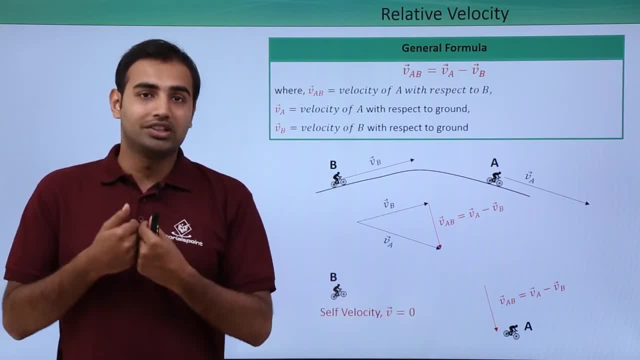 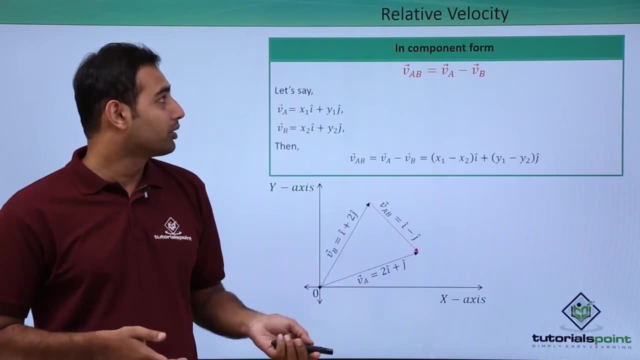 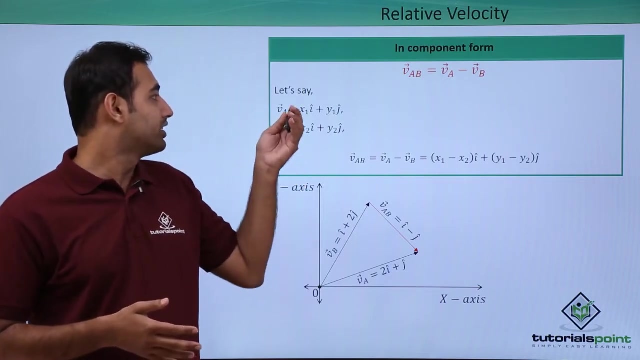 the observer on the cycle B will see. So I hope this fundamental idea about how relative velocity in two dimensions is possible. Now let's talk about the relative velocity when we have been given velocities in component form. So if we have velocity A and velocity B given in component form as x1i plus y1j, 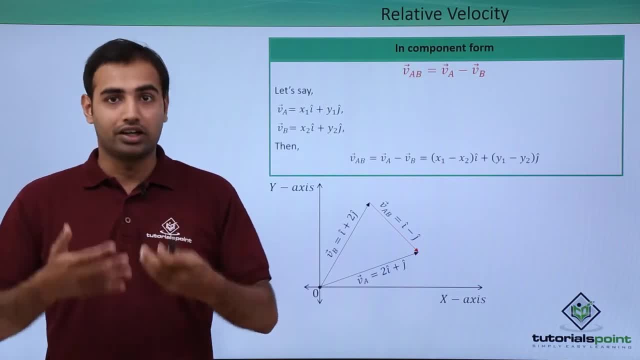 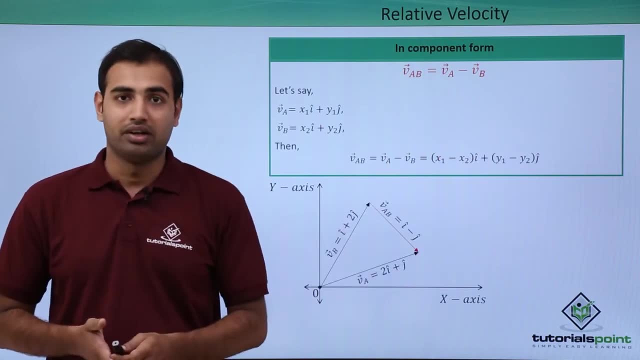 and x2i plus y2j. clearly these two velocities are in ground frame, So velocity of A with respect to B can simply be x1 minus x2i plus y1 minus y2j cap. This is very, very clear. I have simply subtracted the vectors in component form. 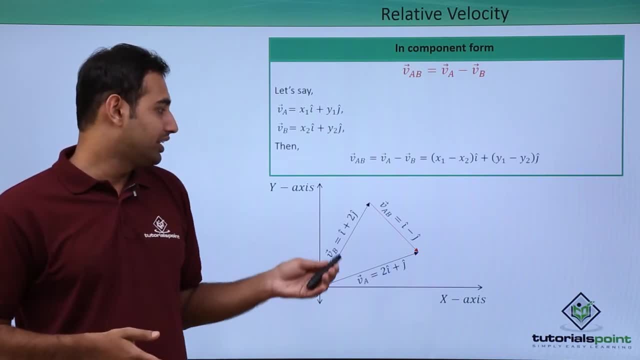 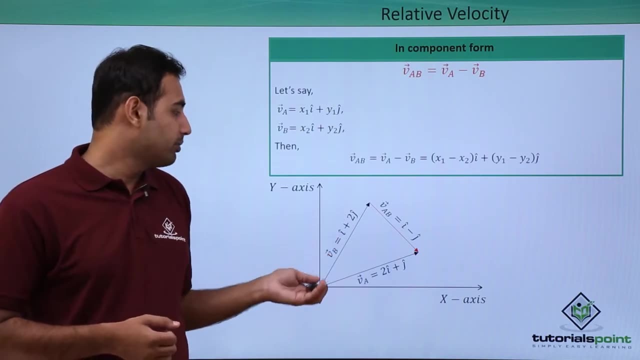 And subtracting vectors in component form is very, very easy. So, taking an example for the same. so if we have VA vector as the value 2i plus j, cap, and if we have VB vector as the value i plus 2j, now if I have to calculate velocity of A with respect to B, then it will. 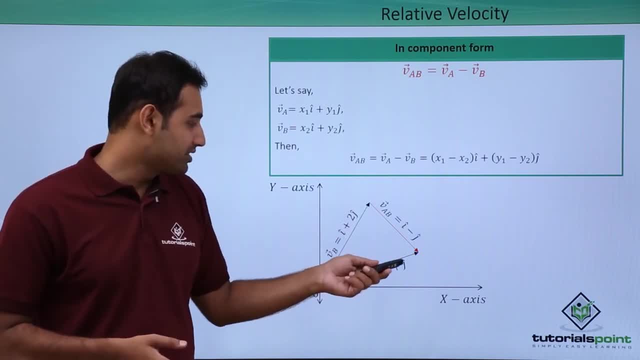 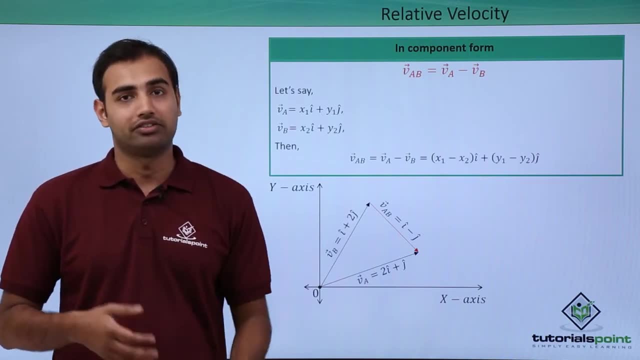 simply be VA minus VB, which will be 2i plus j minus i plus 2j, which will come out to be i minus j. So in component form we can directly draw the vector very, very easily. I hope these ideas about relative velocity are very, very clear to you. 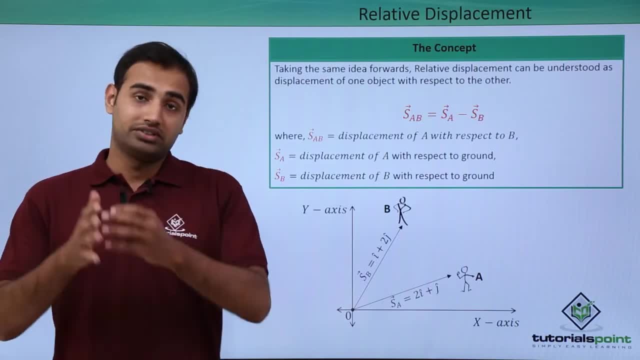 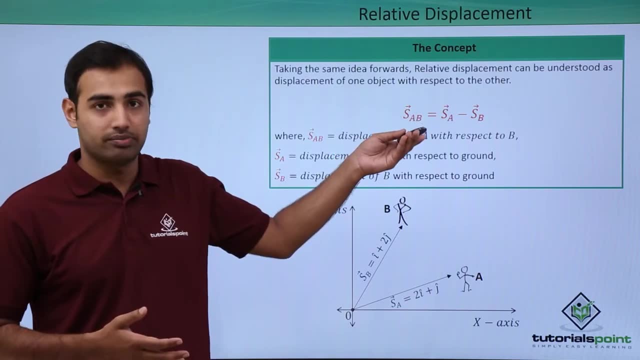 Now let's talk about the concept of relative displacement. Now, just like you learnt in motion, in one dimension the formula for relative displacement will be given as displacement of A with respect to B is equal to displacement of A minus displacement of B. This is also 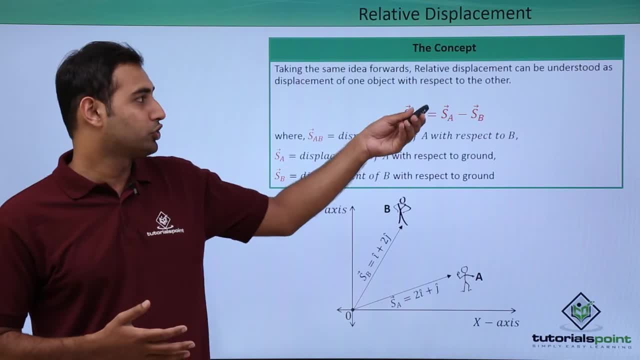 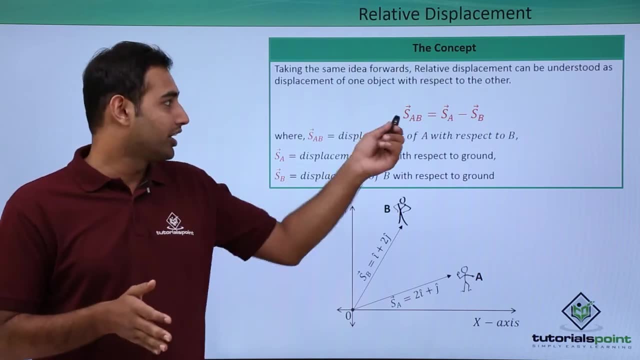 true for position. So position of A with respect to B can also be written as position of A minus position of B. Because position and displacement is very intricately related to each other, We can have the same formula applied for position also. Now, taking an example for the same once. 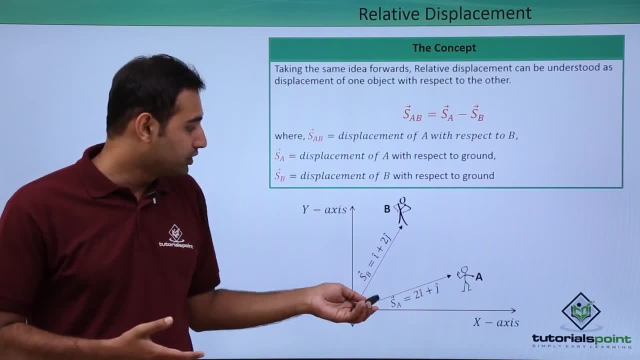 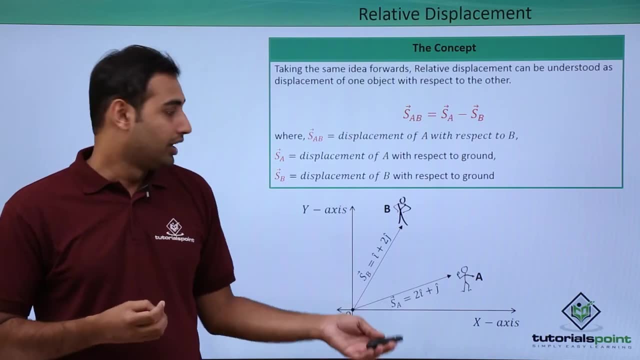 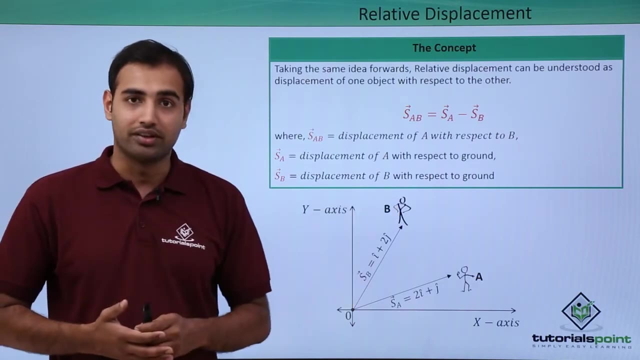 again we have two people, A and B, and A standing at position vector 2i plus j, or I can say that A moved from origin up to a displacement of 2i plus j. Similarly, B has a position vector of i plus 2j, which I can also say that his displacement with from origin is i plus 2j. 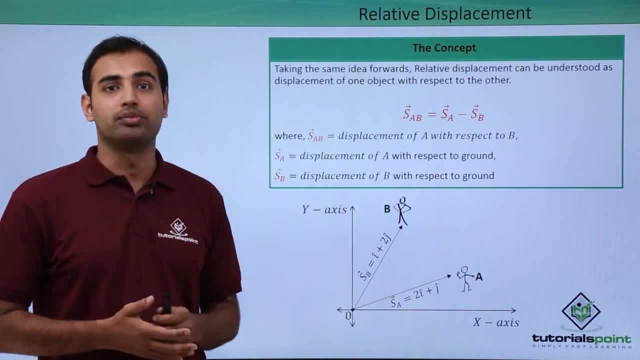 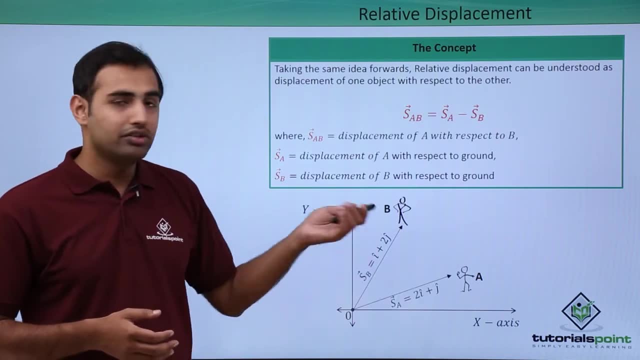 Now, if I have to calculate displacement of A with respect to B, essentially as AB, So I can directly calculate it as SAB, SA minus SB. So SA value is 2i plus j and SB value is i plus 2j. So clearly displacement. 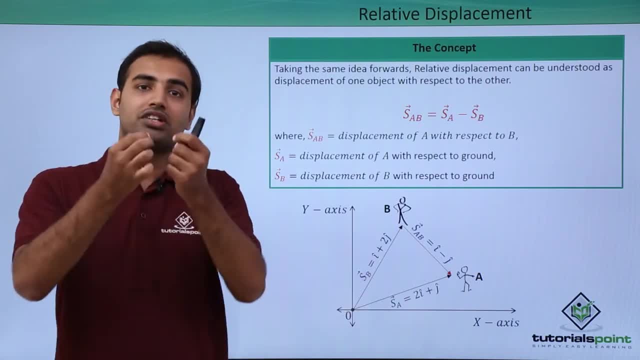 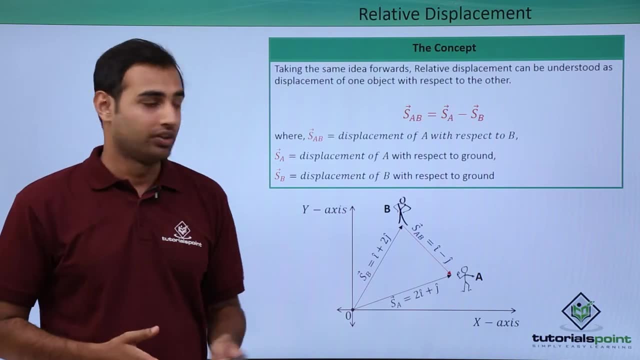 of A with respect to B is i minus j. So what B observes about A, what B observes about A, is that A is standing i minus j cap vector away from himself. So this i cap minus j cap will give me an idea about the magnitude which is clearly square root of 2 here and direction. 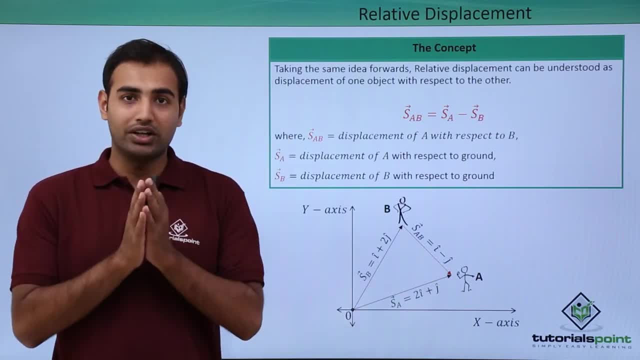 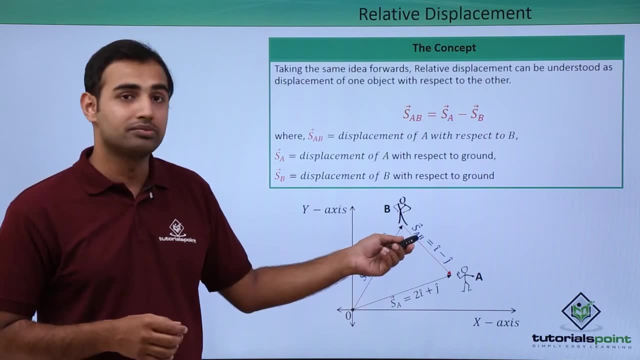 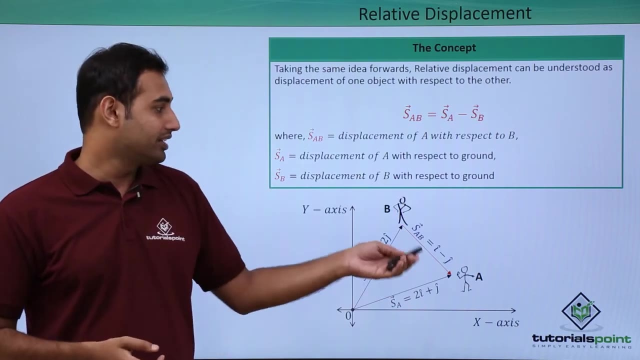 which is in this direction at 45 degree angles. So I hope this concept of relative displacement is also clear to you. Remember, whatever subscript comes later, which in this case is B, is the observer. So whatever result we get, we get that result with respect to that specific observer. So in this case, 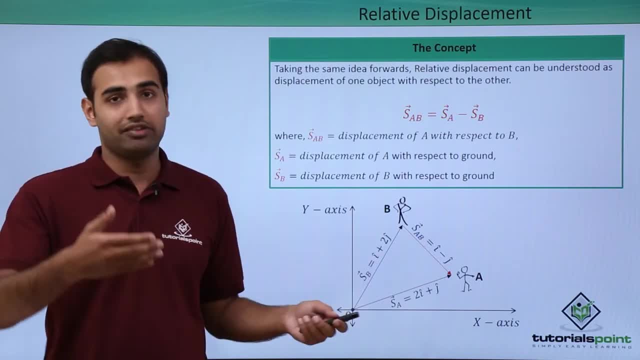 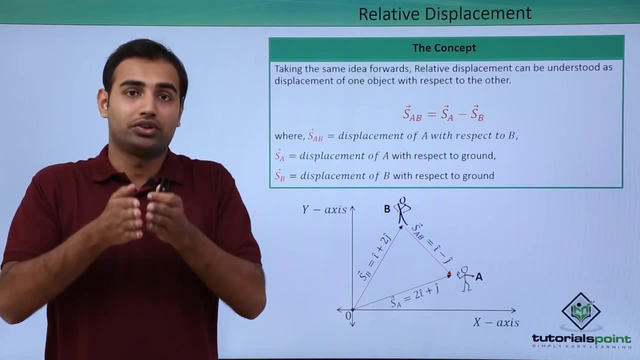 B is observing A having a displacement of i cap minus j cap with respect to himself. So where is A standing with respect to B? or in other words, if B becomes the center or the reference point or the origin, in that case B will observe A to B at this much distance. 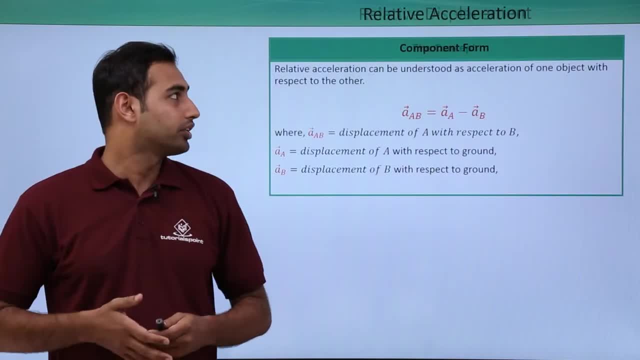 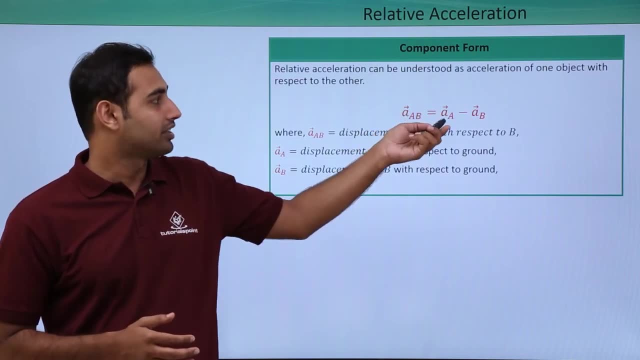 or this much vector away from himself. Now let us talk about the constant. Let us talk about the concept of relative acceleration. On the very same lines, acceleration of A with respect to B can be written as acceleration of A with respect to ground, minus acceleration. 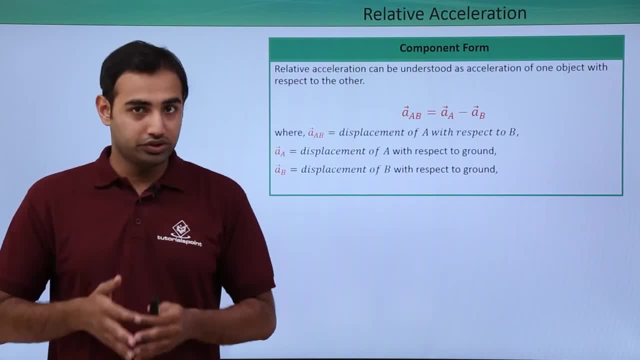 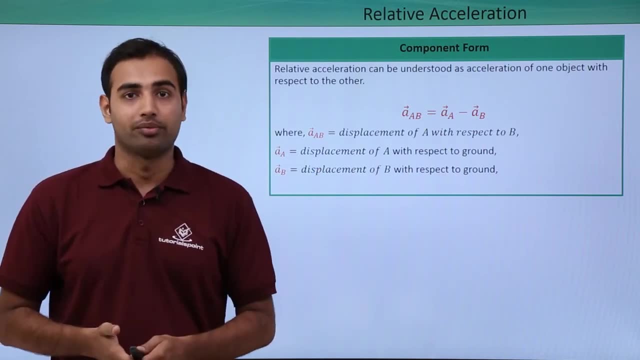 of B with respect to ground. Now, this formula is also something you have learnt in motion in 1D and it can be interpreted in the same way as we have been interpreting the previous two displacement and velocity formulae. Therefore, summarizing what we just learnt, I can say: 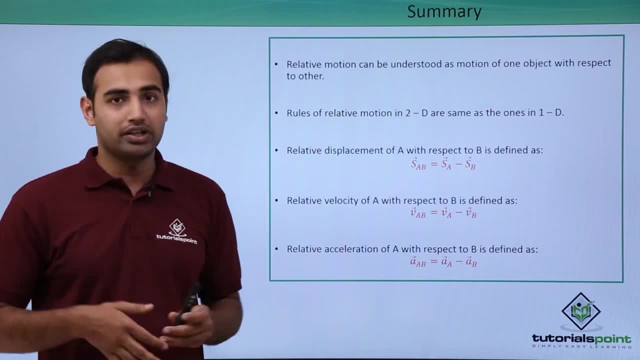 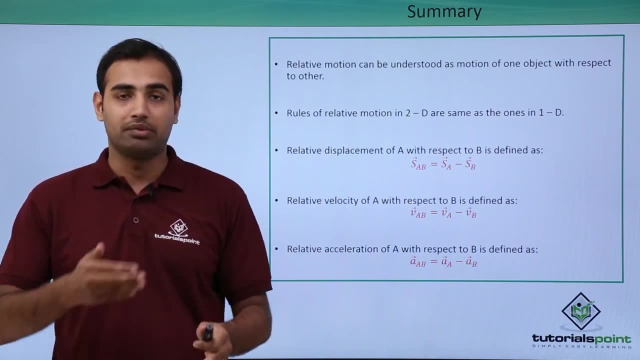 that relative motion can be understood as motion of one object with respect to the other. This is very, very clear Now. rules of relative motion in 2D are same as the rules of relative motion in 1D. I have been reiterating this thing many times. The only point of differences that the vectors.